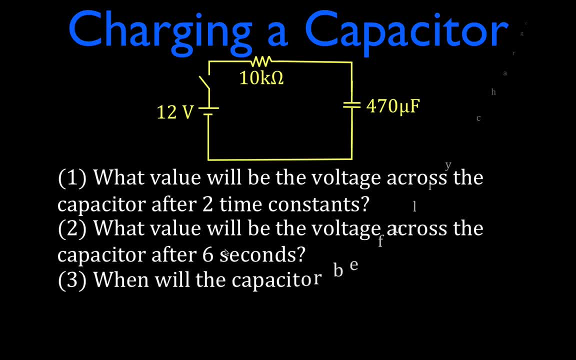 voltage with just regular old time. And then the third thing we're going to do is we're going to determine how long it will take for the capacitor to be fully charged. What does it mean for a capacitor to be fully charged? And then we'll talk about, we'll figure out what will the current 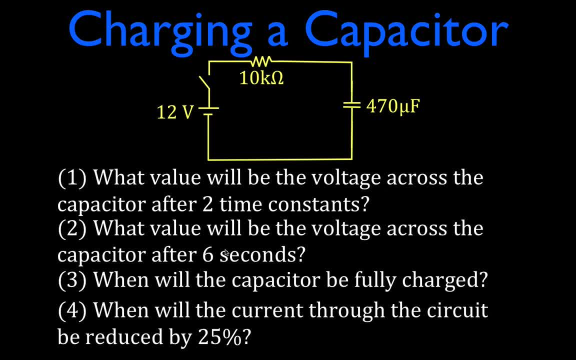 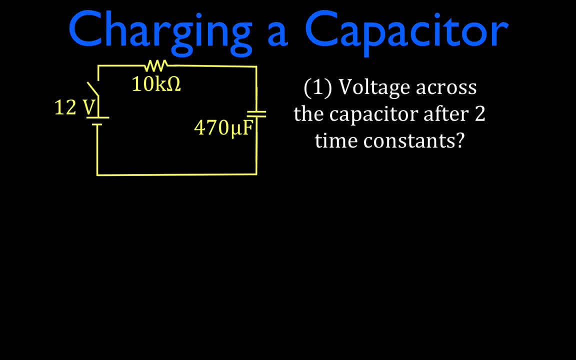 through the circuit be, or when will the current through the circuit be reduced by 25 percent? All right, So the first thing we're going to do is: what is the voltage of the capacitor, across the capacitor going to be after two time constants? Okay, First of all, we have to figure out what 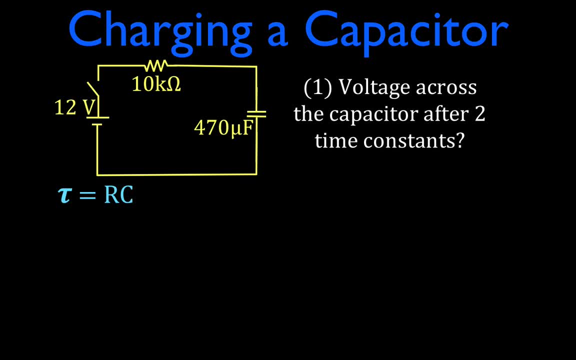 one time constant is The way we calculate the time constant. tau is the symbol we use for the time constant. We just multiply the resistance of the resistor times the capacitance of the capacitor And we get R times C, which is 10 times 10 to the third because of a 10,000 ohm resistor. 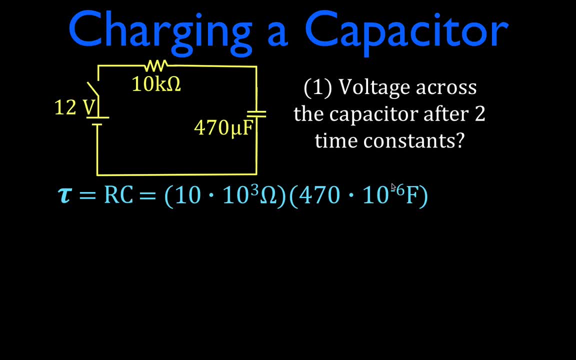 10 to the third ohm And 470 micro 10 to the minus six is micro farads And that gives us that the time constant, one time constant, is 4.7 seconds. We want to know after two time constants. Okay, Now I'm just 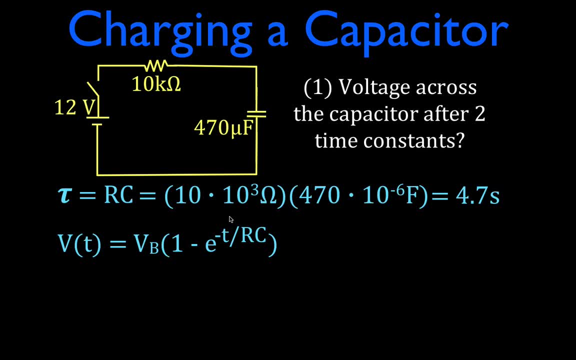 going to get the equation we used to calculate the voltage with respect to time. It's just the voltage of the battery times one minus E raised to the power of minus T over RC. RC is our time constant. That's 4.7 seconds. 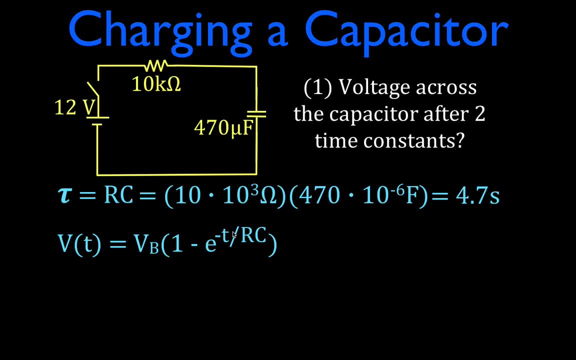 We want to know two time constants. Now, two time constants is obviously going to be 9.4 seconds, And so I'm just going to plug those values in, or plug those two values, in, which is minus 9.4 divided by 4.7, which is obviously two. So we could have just gone here. I wanted to show you. 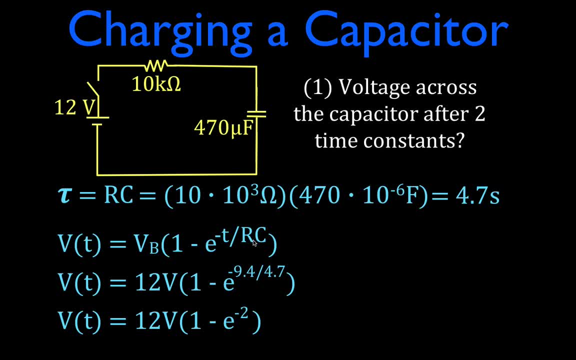 how that works with the time and the time constant, the two time constants. But you see we have 12, which is the voltage of the battery times one minus E, raised to the power of minus two Minus two times constants, And then we can just figure out that that is the voltage with respect to time. 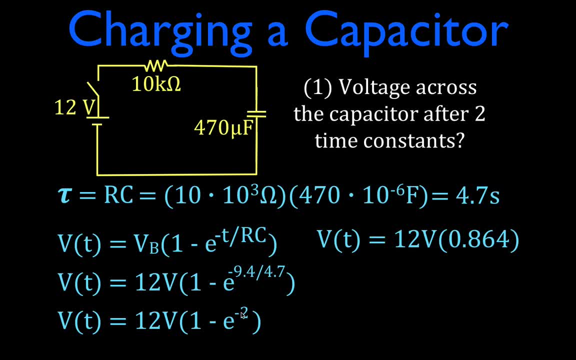 is going to be 12, because that's the voltage of the battery again times 0.864.. Now, if you remember that, after one time constant, the voltage across the capacitor will be 36.36, 63.2% of the voltage. 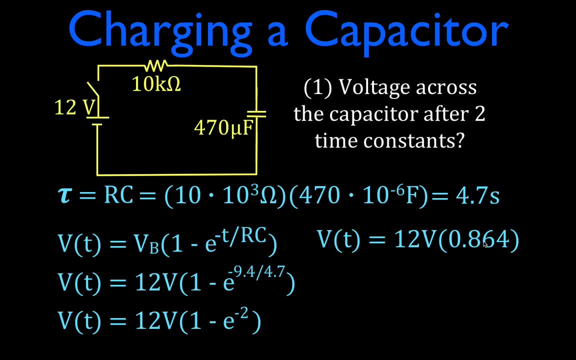 of the source. After two time constants, that's the voltage of the battery, And then we can just constants: it's 86.4.. After three time constants, it's like 95, and then 98.2, and then after five. 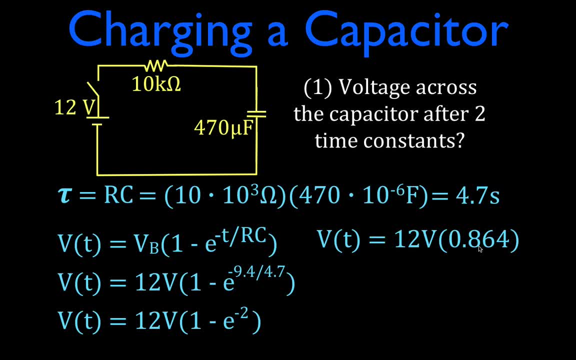 time constants 99.3.. But in this case we have two time constants and you see, that's 86.4% of the source, which tells us that the voltage across the capacitor for this circuit after two time constants will be 10.4 volts. all right, So that's with time constants. 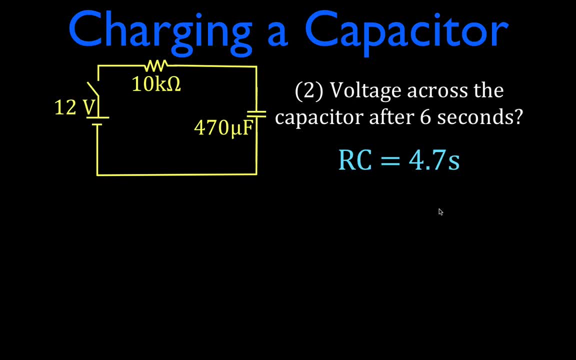 and then the next thing we're going to do is add a specific time. six seconds RC is our time constant again, because we use the same equation: 12 volts for the battery. six seconds T is the time, RC is the time constant, which is 4.7 seconds, and then we get that's 12 times 1 minus. 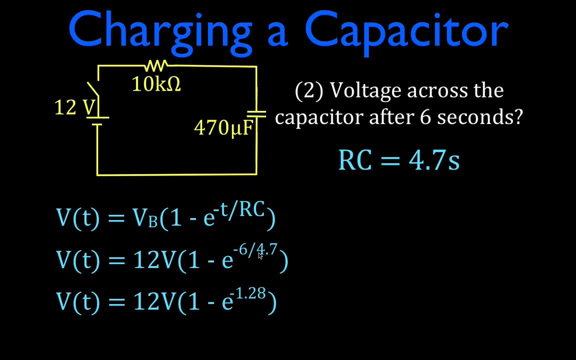 E to the power of minus 1.28, and that tells us that after six seconds, the voltage across the capacitor will be 72.2% of the volts of the source, and that tells us that the voltage across the capacitor at six seconds will be 8.66 volts. 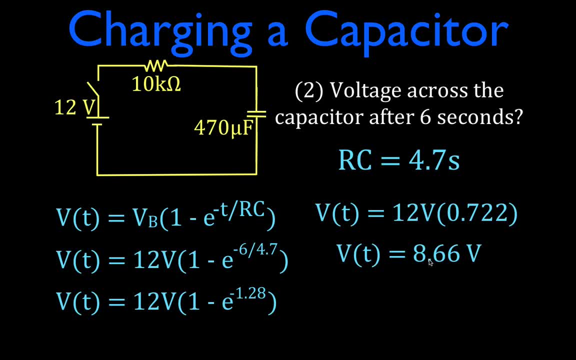 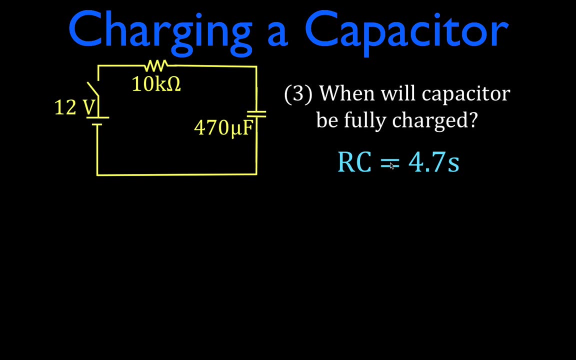 okay, Basically the same thing. whether using time constants or time both time, same equation. okay, All right, now the next thing we're going to do is figure out: say, when will the capacity be fully charged? Here is our value for the time constant Now. 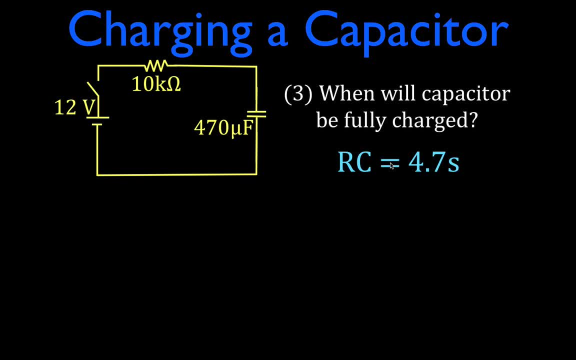 it's generally accepted that the voltage or the capacitor will be fully charged after five time constants. okay, It's an exponentially increasing voltage across the capacitor and after five time constants it's actually charged to 99.3% at the maximum. 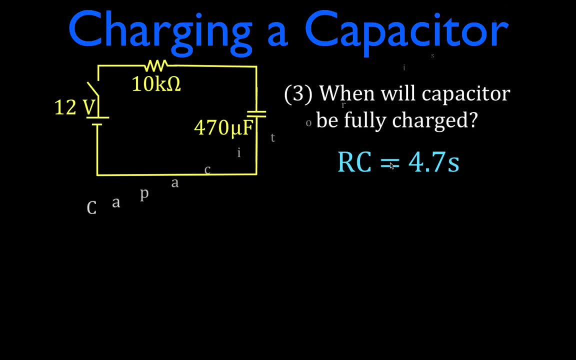 and that is considered to be fully charged. So we're just going to multiply five times the time constant, five times RC. RC is the time constant, again five times 4.7 seconds, and that tells us that the capacitor will be fully charged after 23.5 seconds. okay, 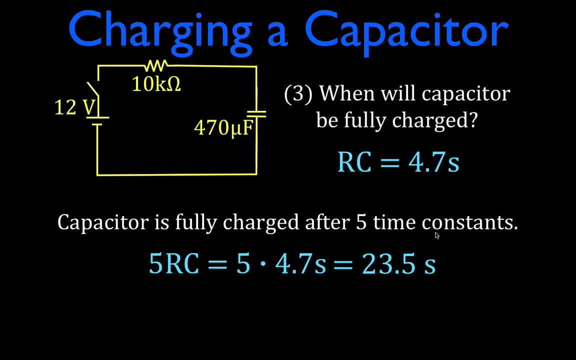 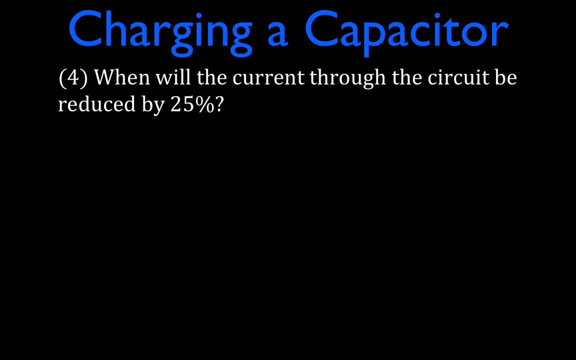 The capacitor is fully charged after five time constants. Okay, and then the last thing we're going to do is we are going to figure out when will the current through the circuit be reduced by 25%? Now, this is the equation we use to calculate the current with respect to time. 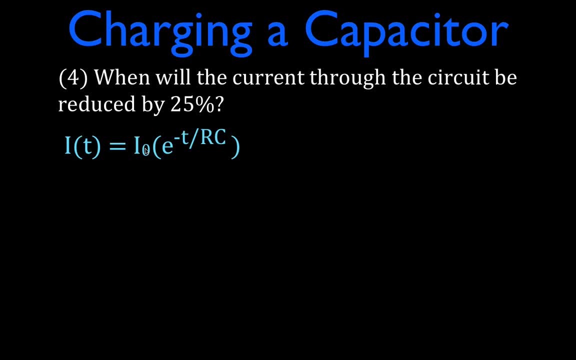 is equal to the maximum current, the initial current, Remember- in a capacitor. when you're charging a capacitor, current goes through its maximum and then decreases exponentially over time. So it's the maximum current times E raised to the power of minus T over RC. 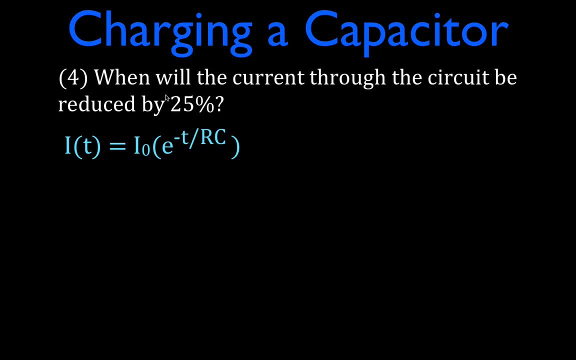 and we actually want to know when will we reduce by 25%? That means we want to know when will the current be 75% of the maximum. So for this term I'm going to substitute in 0.75I0,. that is the maximum current, the initial current, the current at time zero, And so that is 75% of. 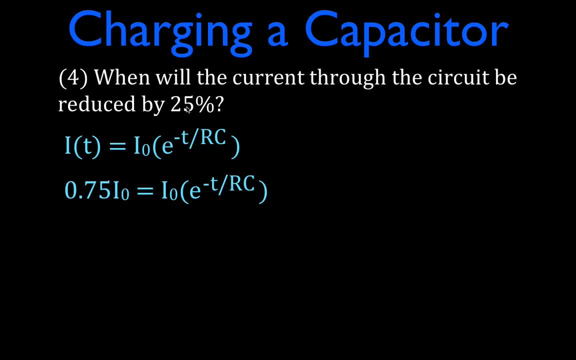 the initial, and that's when it will be reduced by 25%. And then you'll notice I have I0 on both sides, so I can divide this whole equation by I0, and that gives me 0.75 equals E raised to the. 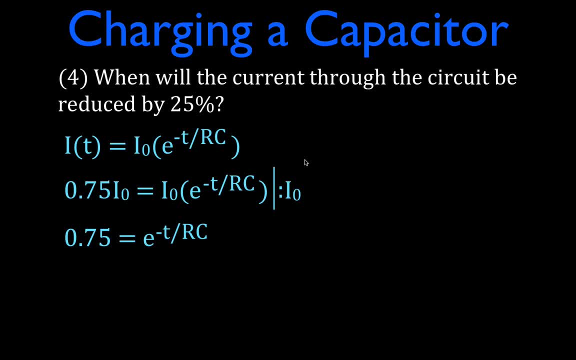 power of minus T over RC. And then the next thing I can do is take the natural log of both sides. Okay, if I take the natural log of E to the X, it's just X. Well, X, in this case is minus T over RC. 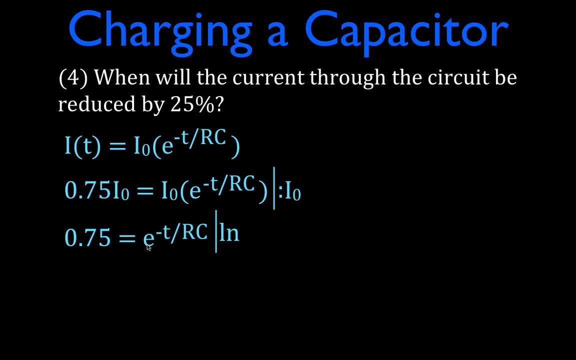 So E raised the natural log of E raised to the power of minus T over RC is simply just minus T over RC. The natural log of 0.75 is minus 0.288, and I'm just going to substitute 4.7 in.